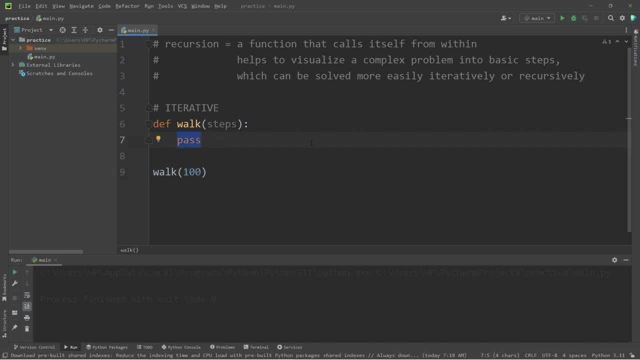 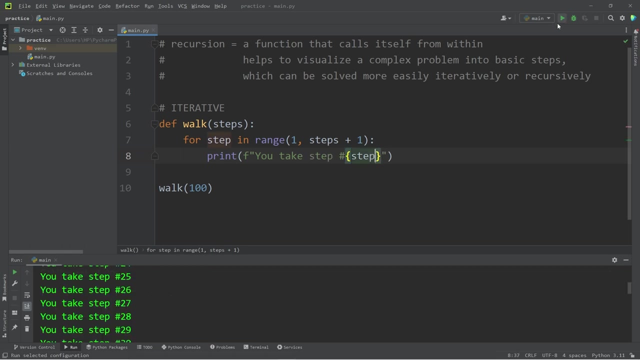 let's say 100 steps. If I were to take an iterative approach within this function, I could create a loop, such as a for loop, For every step in my range, one through steps plus one. I'm going to print an f string. you take step number, step. So that solves our problem. We have taken a single step. 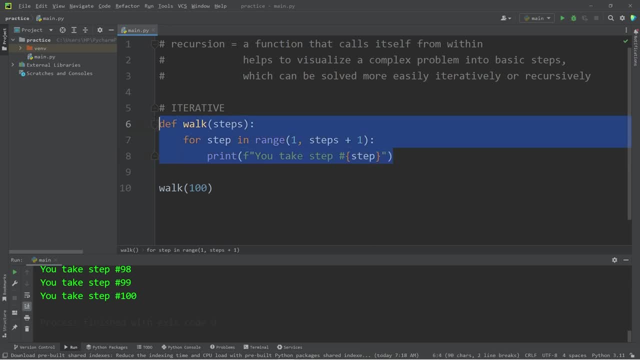 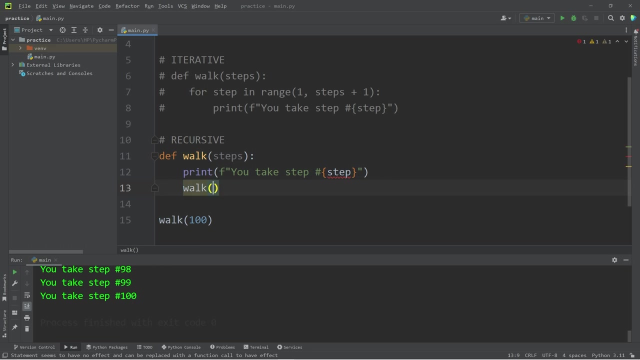 100 times to simulate walking. So that's an iterative approach. We're looping within a function. Now let's take a recursive approach. Recursion involves a function calling itself from within At the end of our function. I'm going to invoke the walk function again, but I will pass. 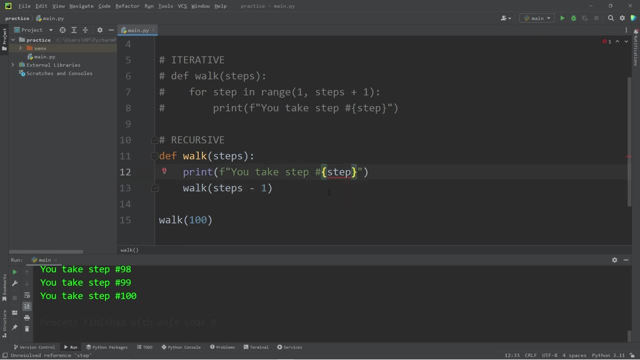 in steps minus one. Let's change step to steps. We're invoking this function from within. It's creating a loop, but we will include the function itself, Whereas in with iteration, we're looping only within the function. Let's see what happens. 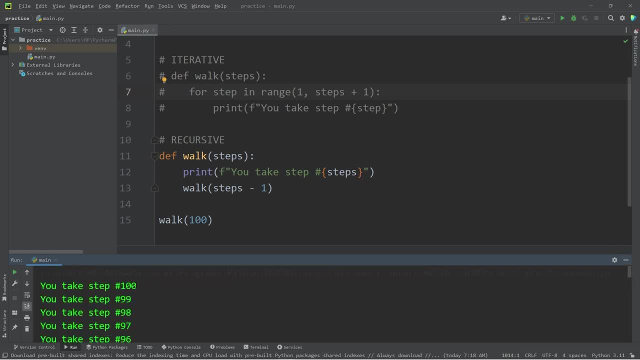 Recursion error. Maximum recursion depth exceeded. This time we're beginning at 100.. We're iterating downwards and we're going below zero. We don't want to take negative steps. We need what is known as a base condition. When do we want to stop? I'm going to add one line. 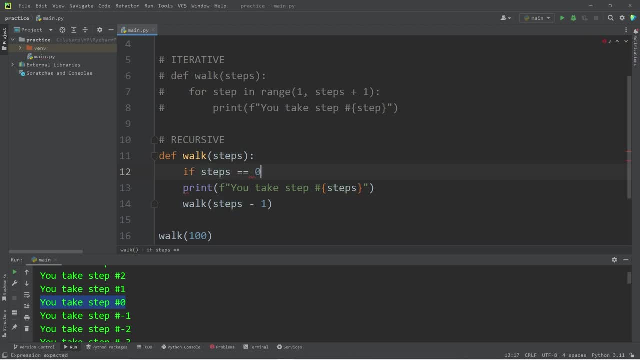 If steps is equal to zero to exit a function, you can return. Let's try that again. That's much better, but we're counting. I would like to count up. I'm only going to print the number of steps after we invoke the walk. 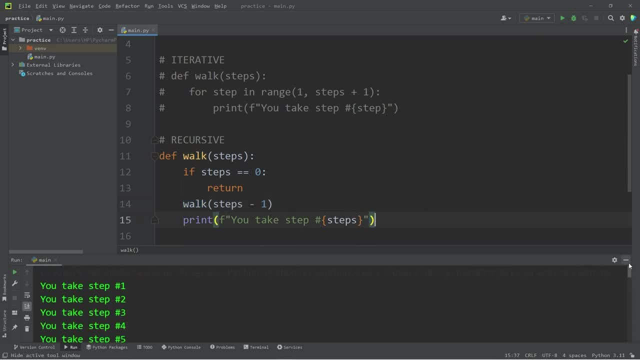 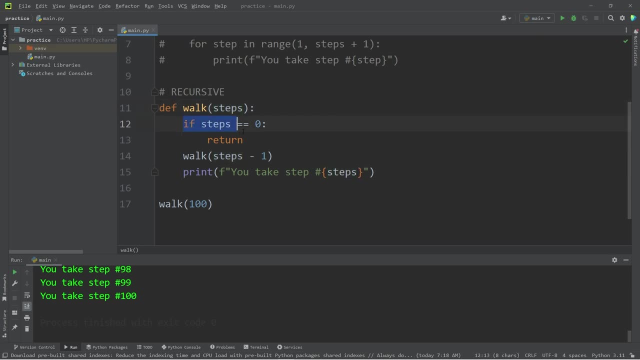 function. Okay, that solves our problem. So how does this work exactly? When we enter the walk function, after accepting a number of steps, we check our base condition, Then we invoke the walk function again, but pass in one less than the number we originally accepted. In a way, we're 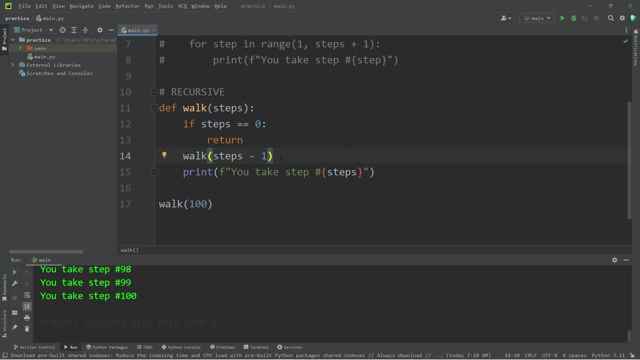 creating a loop, but we're involving the function itself. When you invoke a function, you're going to add what is known as a frame to the call stack. There is a certain order in which we resolve functions. It's a stack data structure. You start at the top and work your way down. It's like a 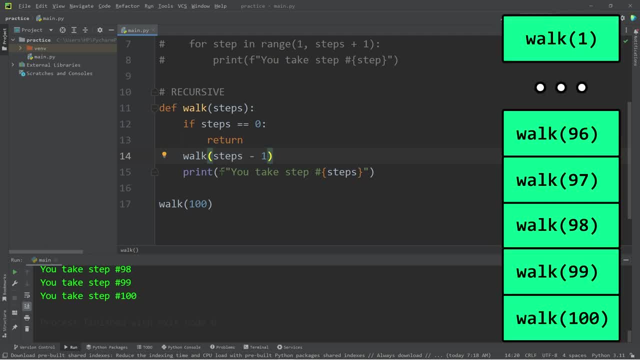 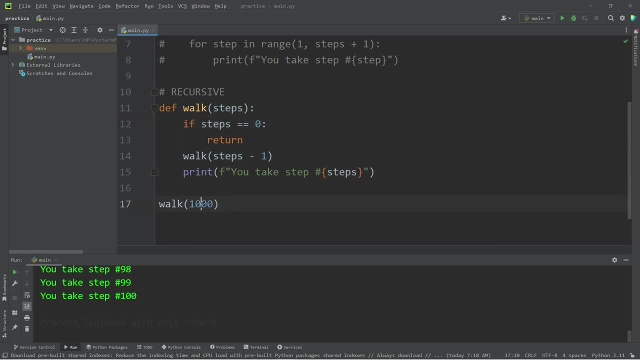 stack of CDs or movies. We add frames to the call stack until our condition is met. Then we undo everything, starting at the top. If you have too many frames on the call stack, let's walk a thousand steps. This is what would happen. Recursion error. Maximum recursion depth exceeded. There's a limit. 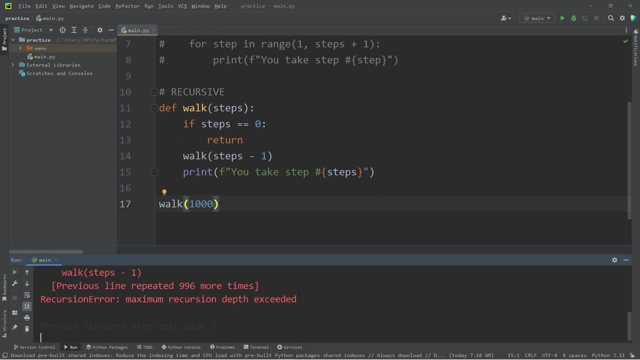 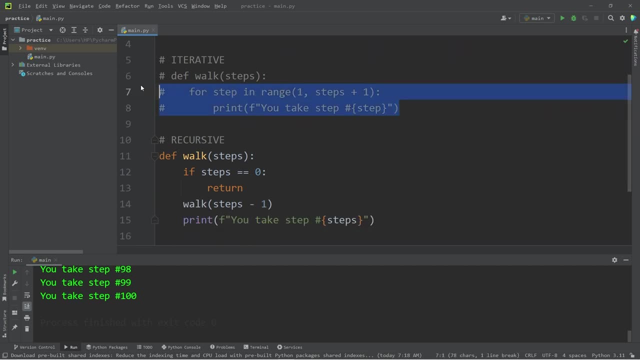 to how many frames can be on the call stack. That's an issue to keep into consideration. You can solve many problems, either iteratively or recursively. For a problem such as this, I would stick with an iterative approach. A recursive approach tends to be slower than an iterative approach, but at times 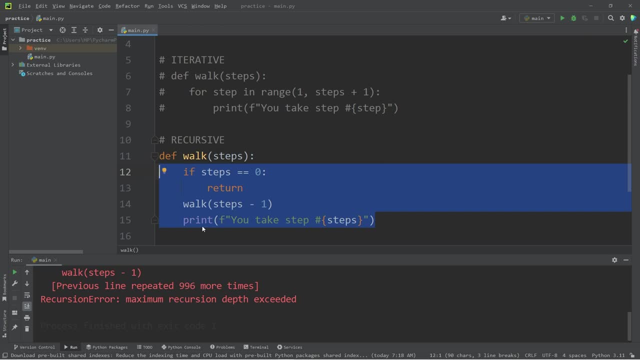 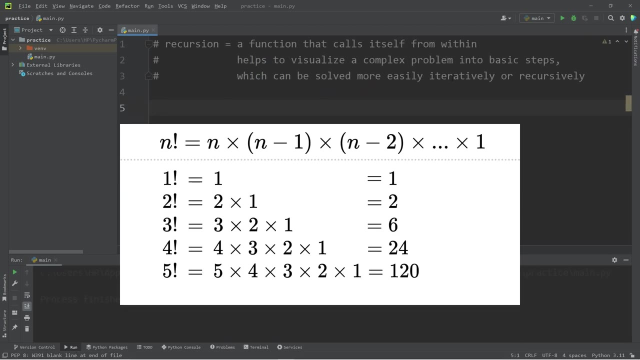 it can be simpler to write, which you'll see in data structures and algorithms. Recursion is going to be your best friend. Let's take a different approach. We will find the factorial of a number, both iteratively and recursively. I will define a number with a factorial of a number. I will define. 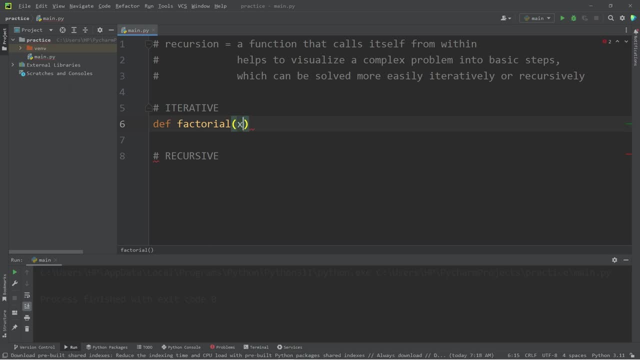 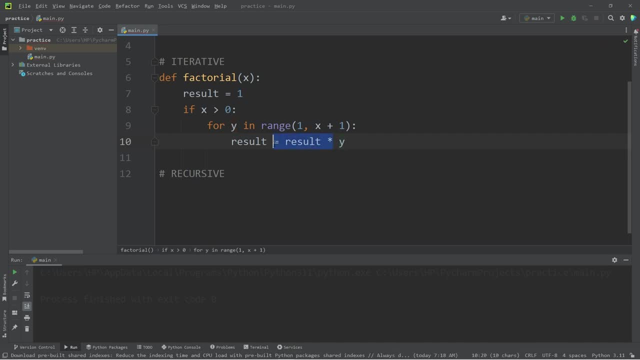 greater than 0. with my for loop at x, I will return y equal to result times y. We could simplify this to result times equals y. Then, outside of the for loop, I will return whatever the result is. Let's invoke the factorial function and pass in a number like 10.. Then I will print whatever is. 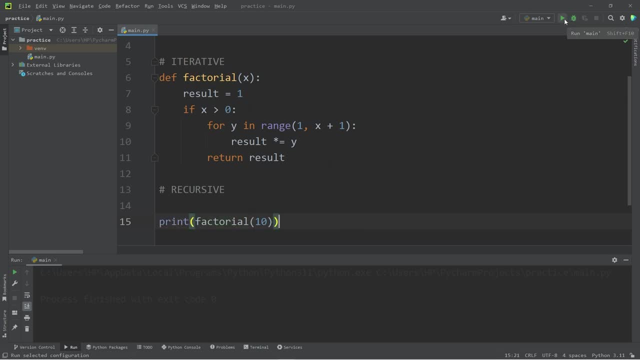 returned. Factorial 10 is 3,628,800.. If I was to take a recursive approach完了, weekends will take the iteration as 2.. You have to keep track of whether it is a neutral term or not. We state.